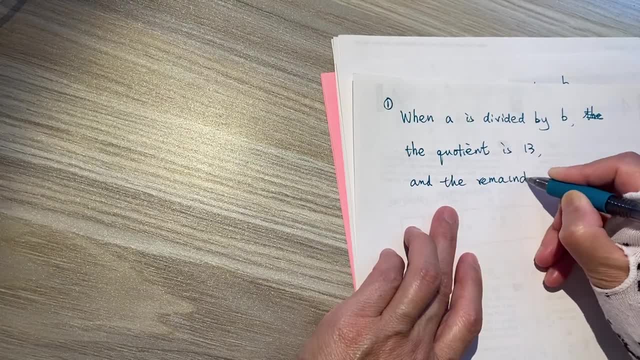 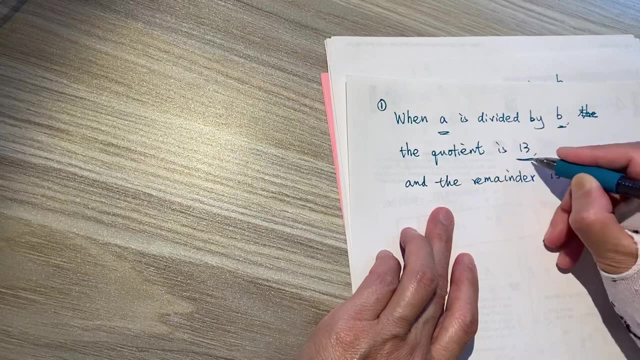 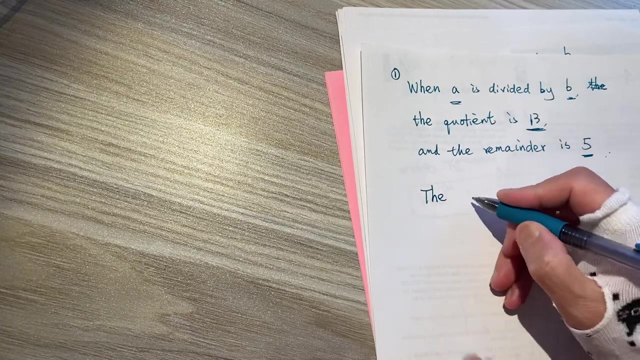 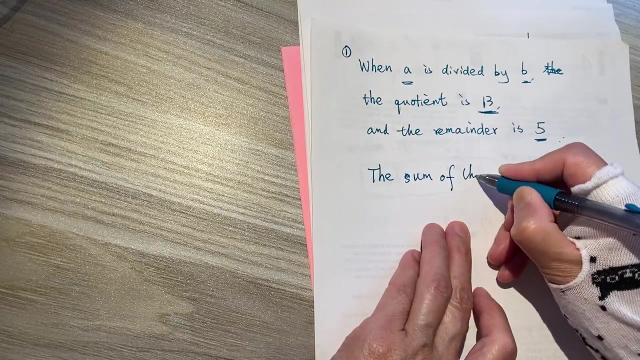 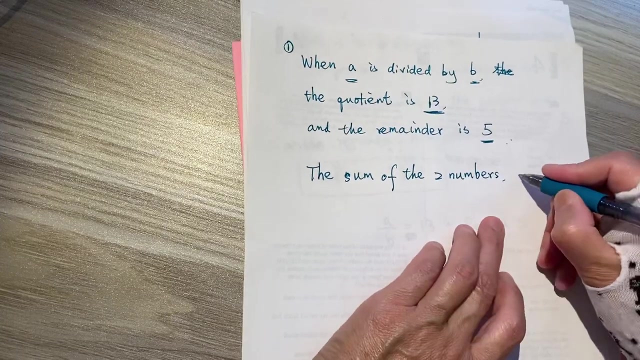 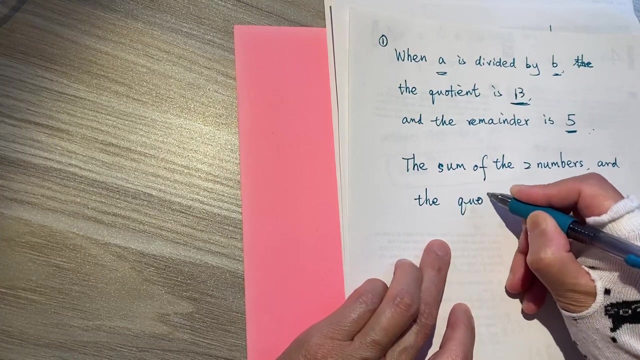 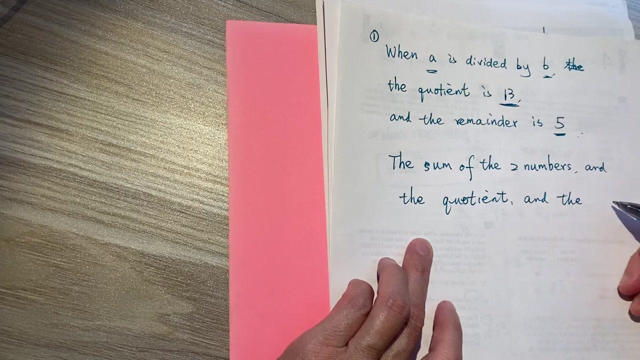 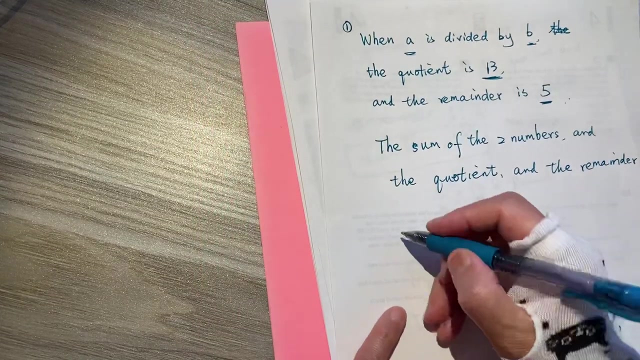 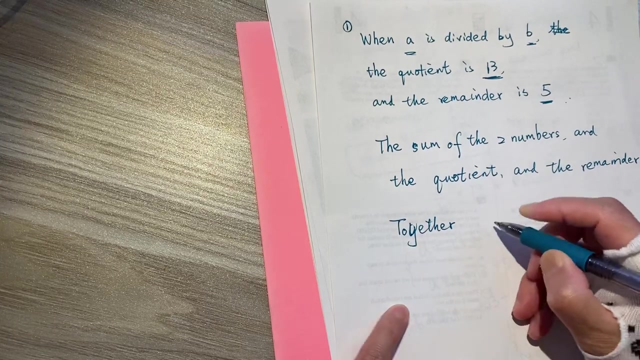 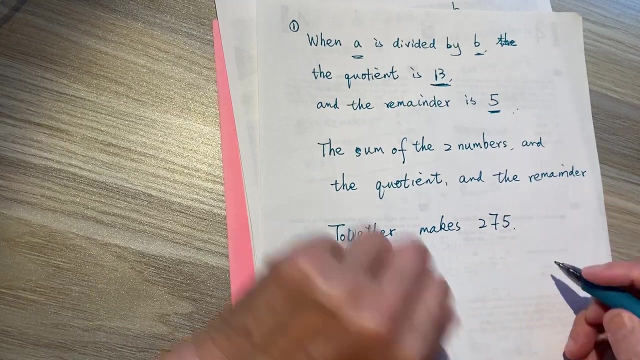 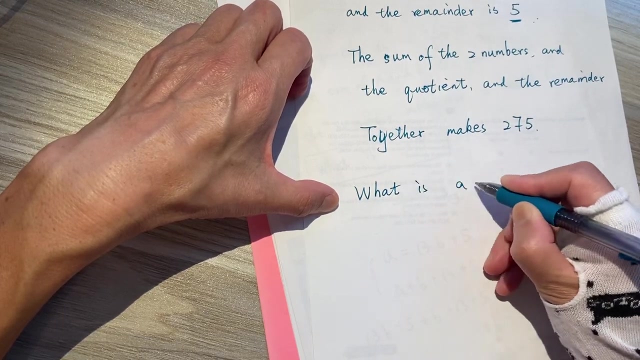 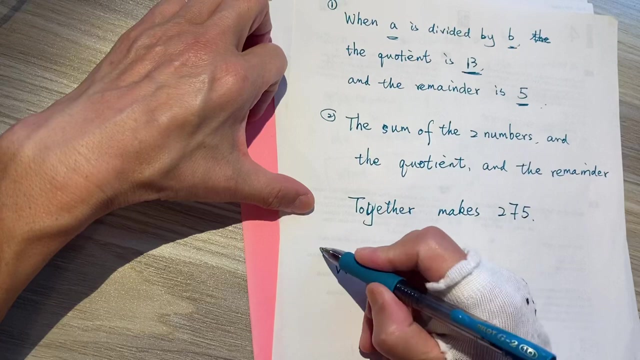 The sum of the two numbers is 5.. The sum of the two numbers And the quotient And the remainder Together, Together Maybe 6,275.. What is A? What is the number A? Okay, so when we see this, we have three components. 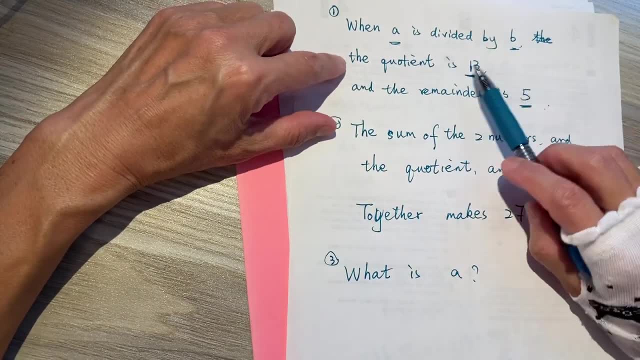 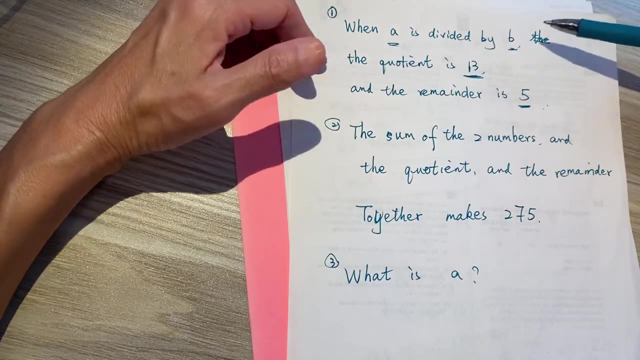 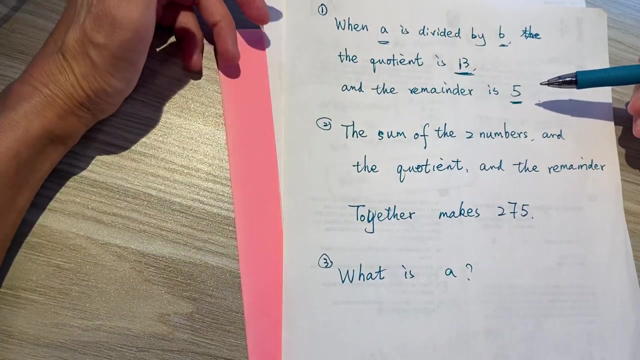 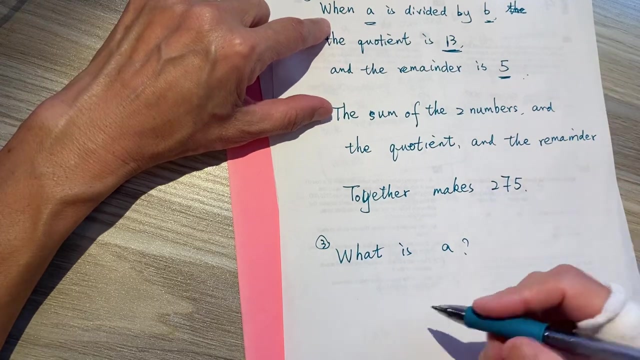 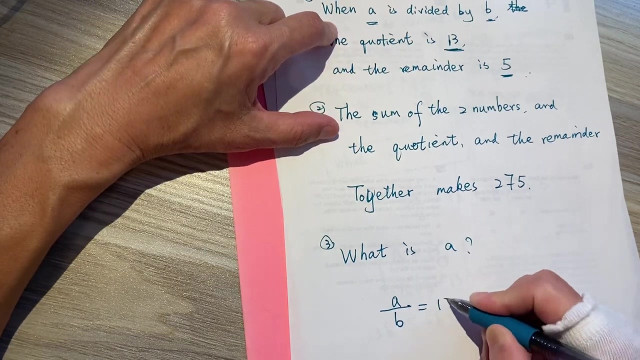 The first: when A is divided by B, the quotient is 13 and the remainder is 5.. So We need to translate this sentence- English sentence or real human language- into machine readable or mass readable equation. So the first sentence we can get when A is divided by B, A divided by B equal to 13 and plus a remainder of 5.. 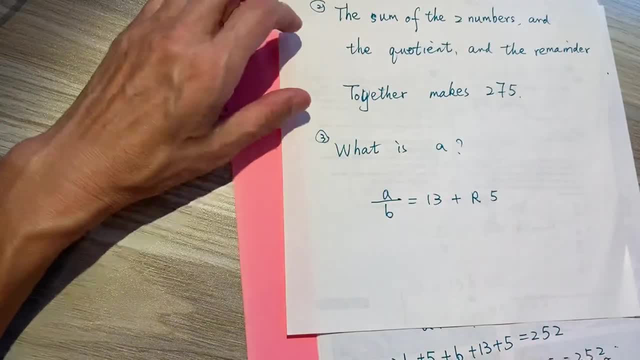 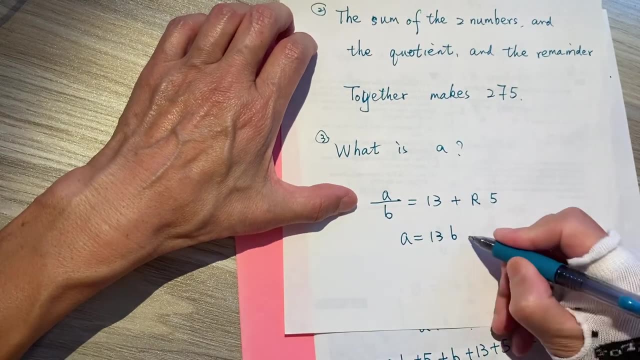 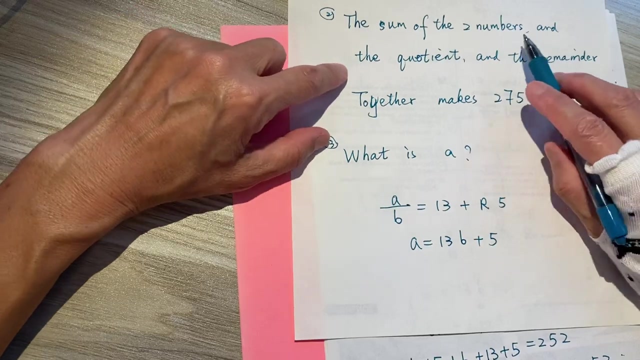 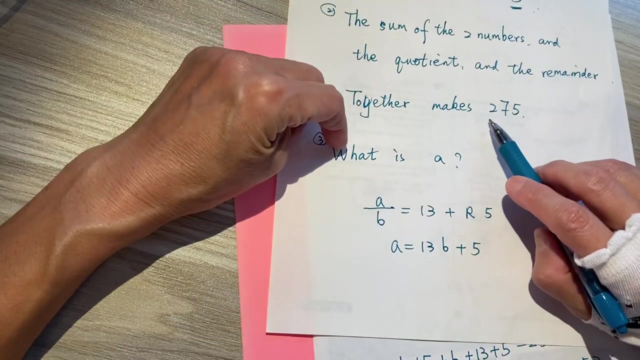 In another way we can write it instead of this fraction form We can write as: A is 13 times of B plus 5. It's even more than 13 times of B, And the sum of the two numbers of A and B and the quotient and the remainder four numbers together makes make not as sorry. 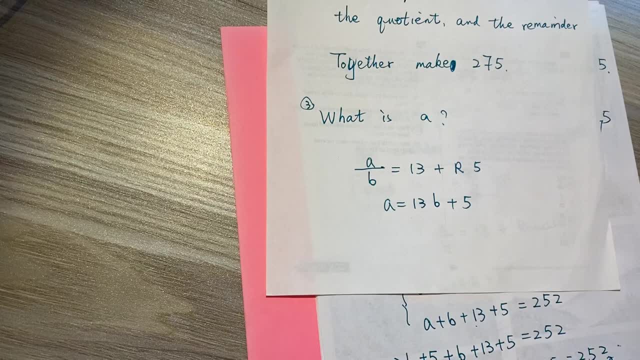 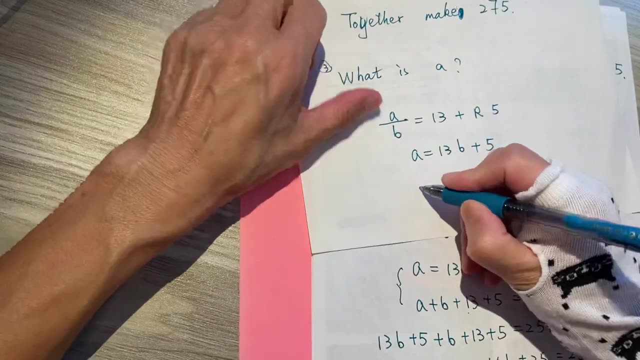 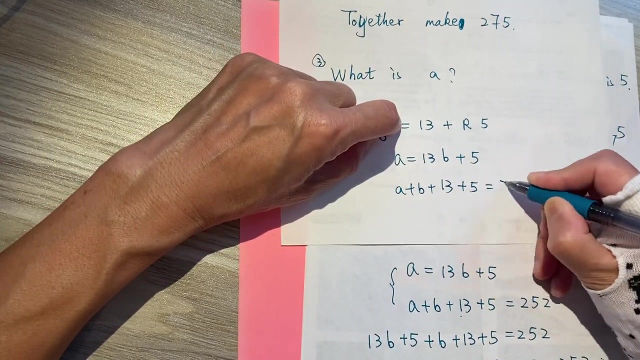 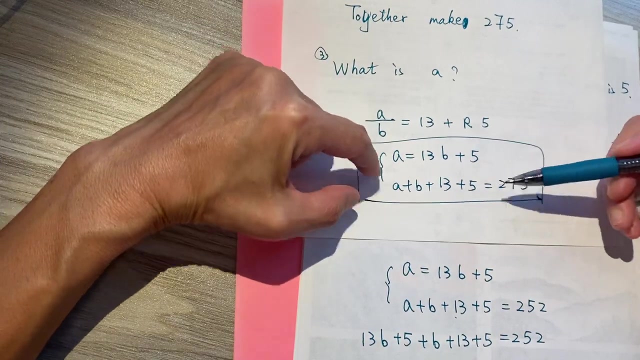 When you do math, you need to care about grammar, or when you do anything, 275.. So A plus B plus 13,, the quotient plus 5, the remainder 275.. So now we get this equation. This question has two variables. 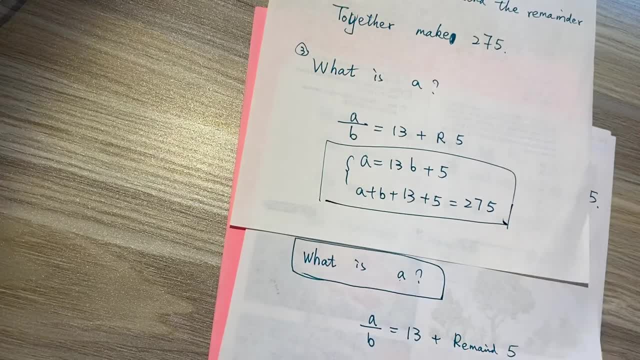 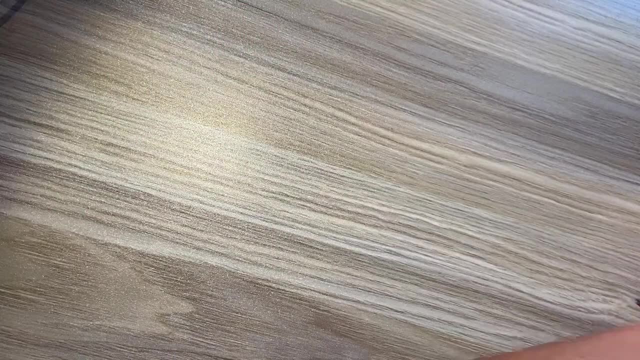 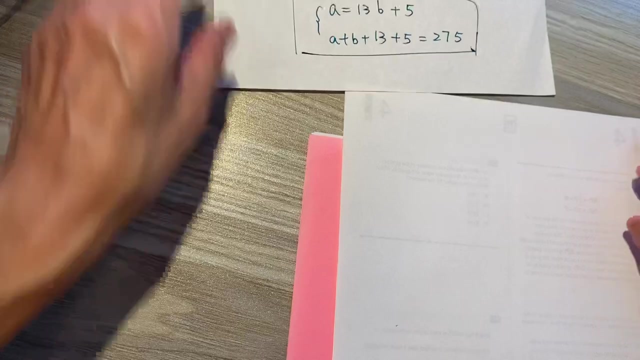 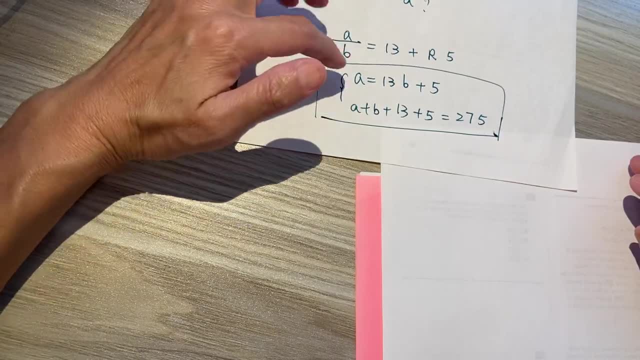 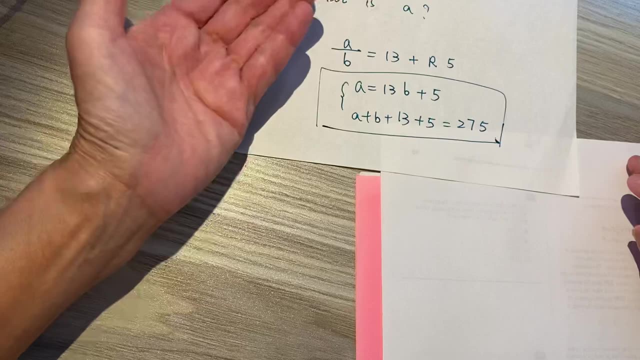 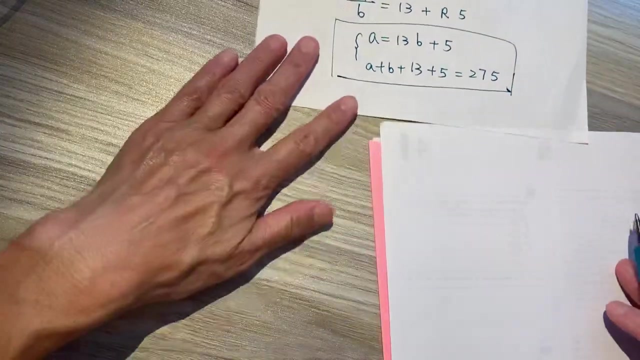 We want to find A, So A is complicated. We can substitute A with B, So figure out B and then plug back back in Into this function. we can figure out A right, Okay, So A is this equation, this part. 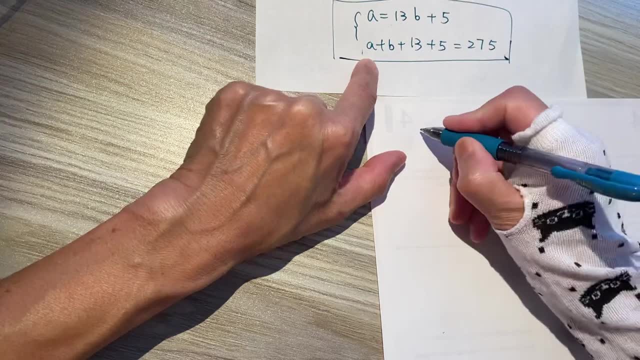 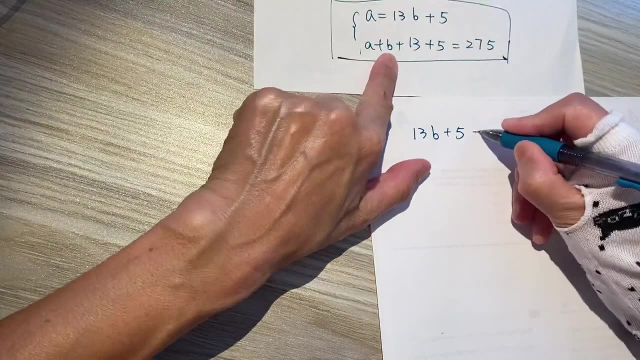 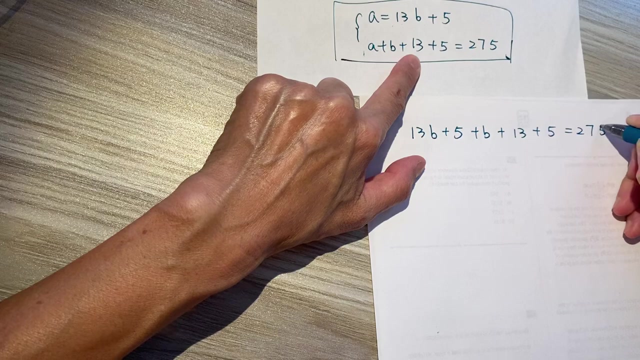 We will substitute A with 13B plus 5.. So 13B plus 5, this is A plus B plus 13, plus 5 equal to 275.. So 14B equals- uh-oh, I am a little bit out of the range. 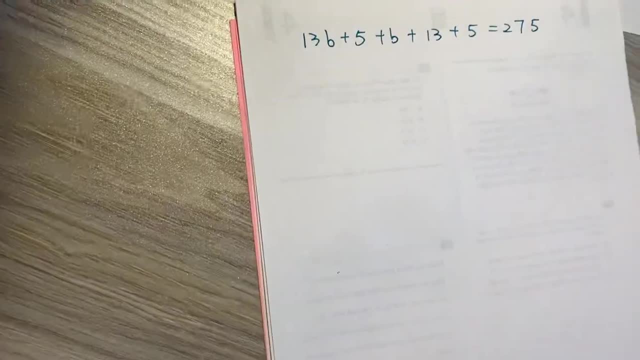 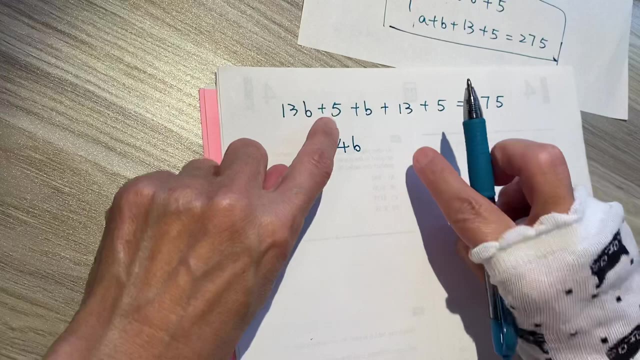 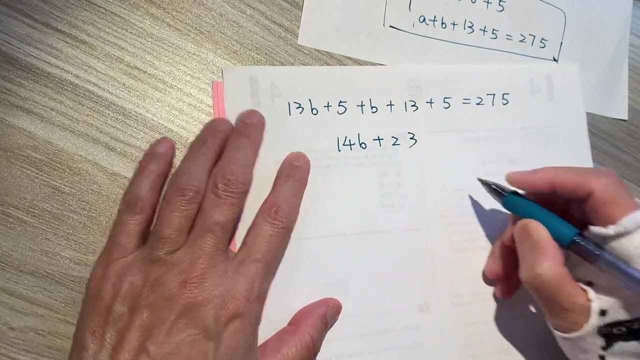 Okay, Are you seeing what I am seeing? So 14B, 5,, 10,, 13,, 23,, plus 23 equal to 275.. So 14B, 5,, 10,, 13,, 23,, plus 23, equal to 275.. 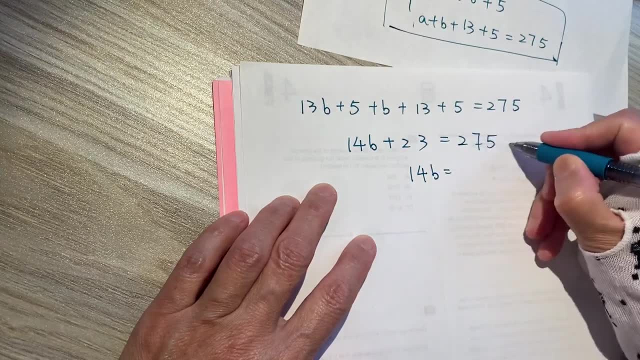 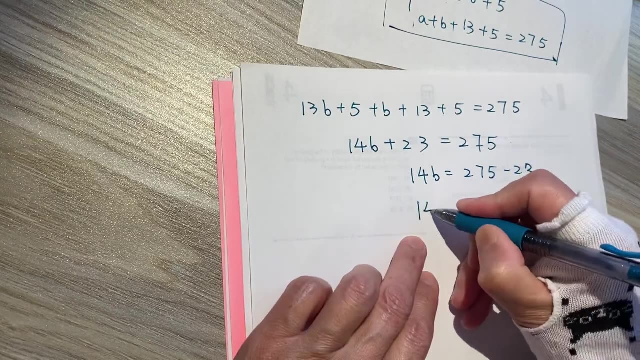 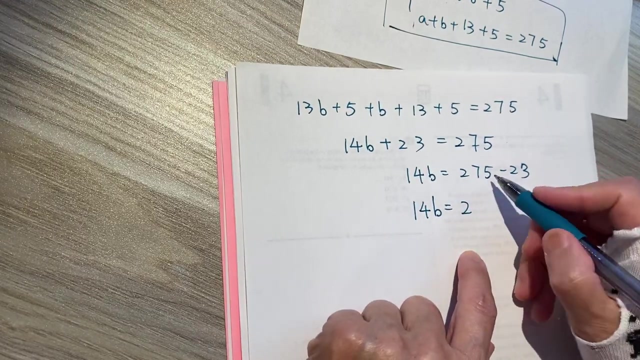 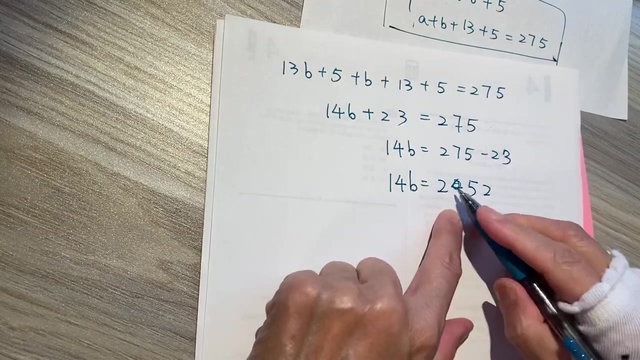 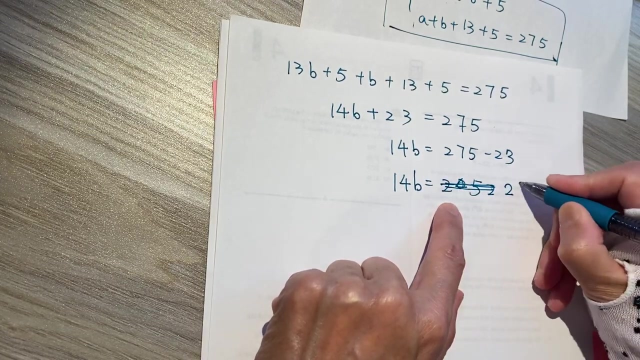 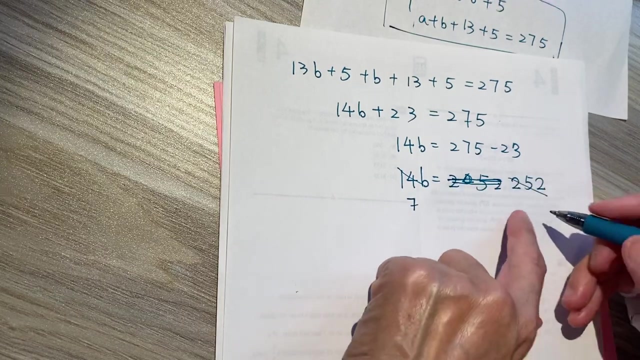 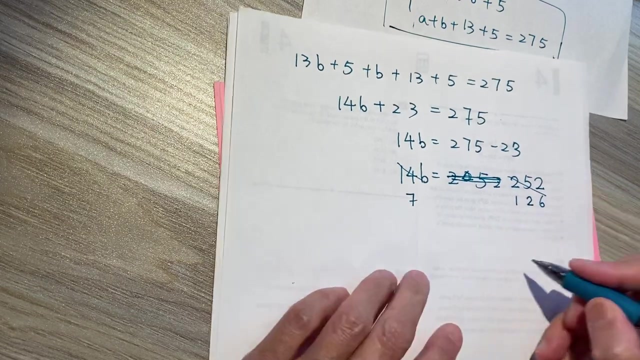 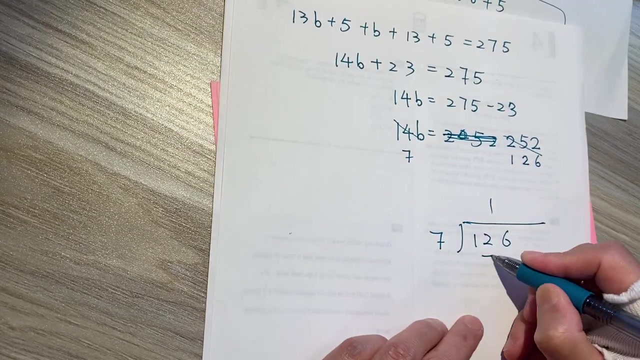 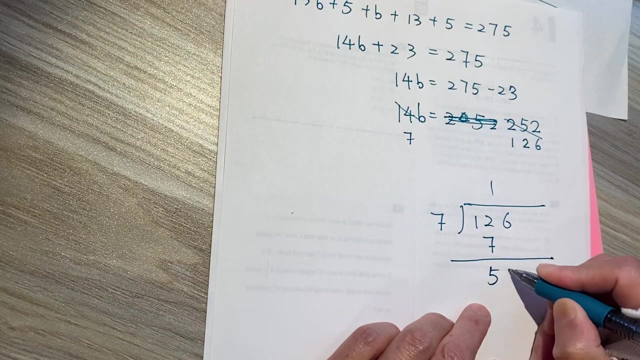 So 14B equal to move to the right, So 14B equal to move to the left. Move it here: so 275 minus 23,. so 14B equal to 252.. So B divide 7, 1, 2, 6, 126 divided by 7, 177, and 56, 7856, 56.